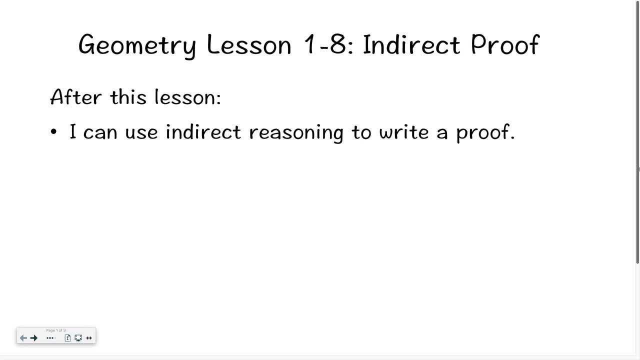 Hello class. welcome to Geometry Lesson 1-8,, which is all about indirect proofs. After this lesson, you should be able to use indirect reasoning in order to write a proof. Before we get started on this lesson, I want to do a quick shout out to Lizzie. 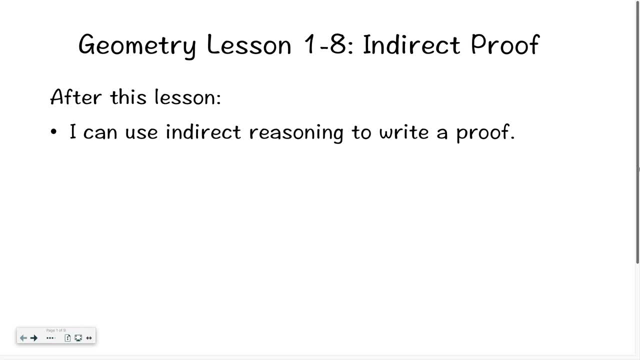 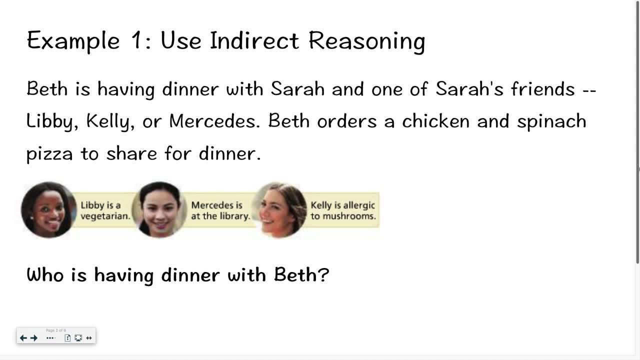 She just stopped by to say hi right before I started recording. Alright. example one: use indirect reasoning. Okay, so let's talk through this situation and figure out how to use indirect reasoning. Indirect reasoning is going to sound a little. the name itself sounds a little scarier than what it actually is. 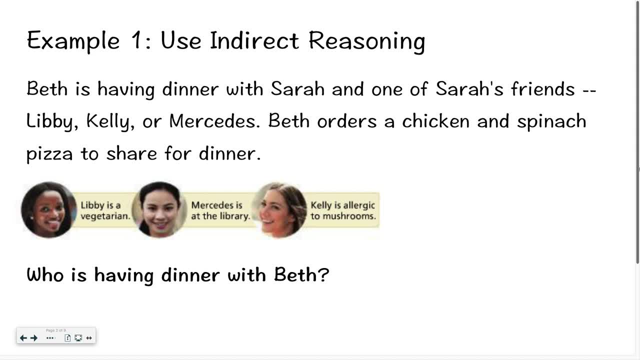 You guys naturally already do this kind of thinking. Okay, so Beth is having dinner with Sarah and one of Sarah's friends, Libby, Kelly or Mercedes Beth, orders a chicken and spinach pizza to share for dinner. Who is having dinner with Beth? 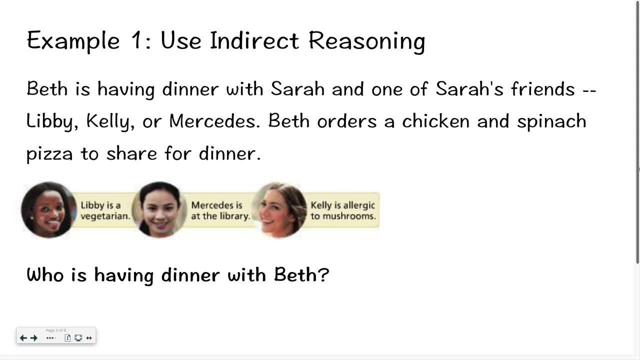 Okay, and then it gives us three pictures and descriptions of Libby, Kelly and Mercedes And information about each of them. Okay. so if we look on the left hand side, Libby, it says, is a vegetarian. Okay so if Beth ordered a chicken and spinach pizza to share for dinner, would Libby be someone that's present? 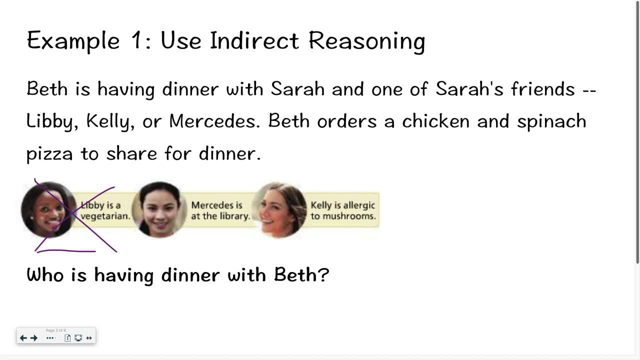 No, because she's a vegetarian, She's not going to eat the chicken. Okay, let's look next. We have Mercedes. Mercedes is at the library, So if she's at the library, does that mean is she able to be at dinner? 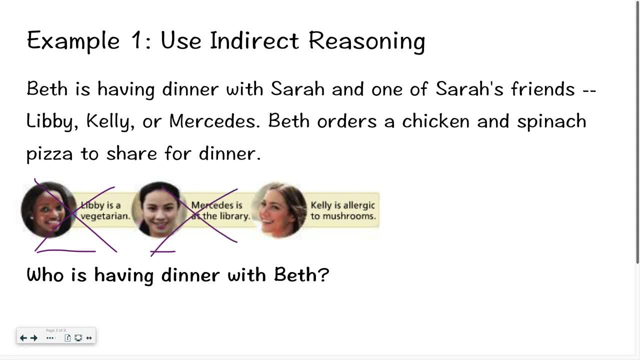 No, So we're going to cross Mercedes off the list. Kelly is allergic to mushrooms. Okay, so is Kelly able to eat a chicken and spinach pizza? Yes, So you'd say Kelly is having dinner with Beth. So that's all. it is just kind of using that process of elimination. 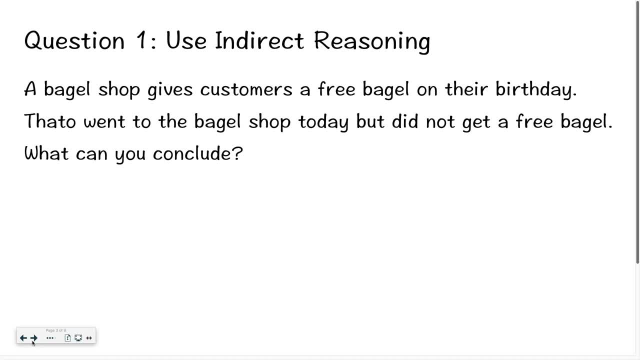 So I want you to use indirect reasoning on this first question. A bagel shop gives customers a free. A bagel shop gives customers a free bagel on their birthday. They don't went to the bagel shop today, but did not get a free bagel. 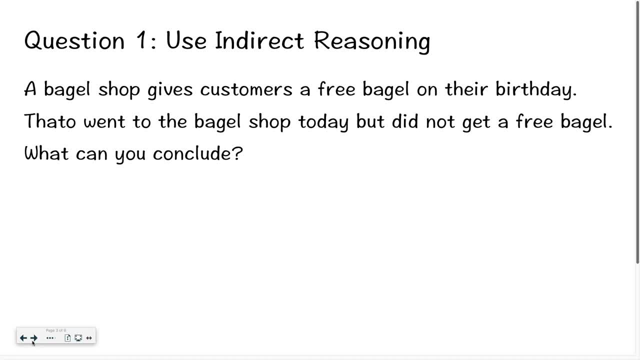 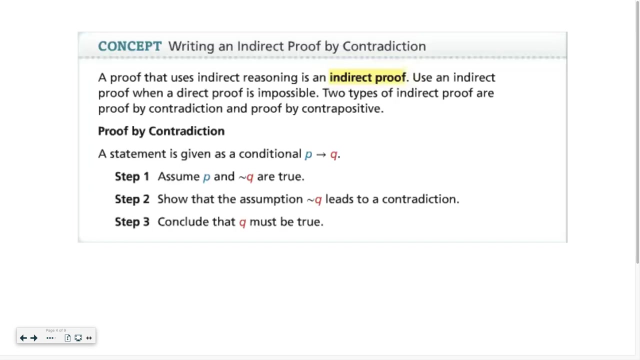 What can you conclude? Hopefully, you concluded. Hopefully, you concluded that it is not Thato's birthday and that's why he didn't get a free bagel. All right now, take a screenshot of this, because it's going to be something really important. 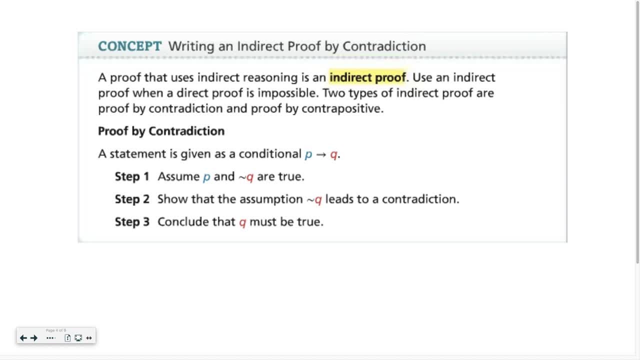 Writing an indirect proof by contradiction. So a proof that uses indirect reasoning. what we were just doing is an indirect proof And in order to To write an indirect proof, you only want to do that when a direct proof is possible. So meaning, if there are so many correct answers that you can't possibly go through and prove that each correct answer is correct. 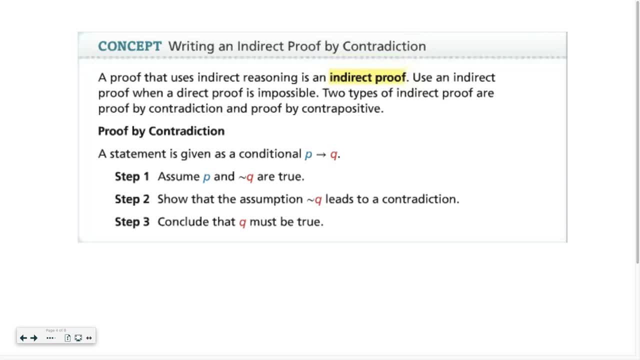 you use indirect proof instead, And there are two different types of indirect proofs: One is proof by contradiction and the other is proof by contrapositive. So first we're going to talk about proof by contradiction And a proof by contradiction, The really, really important. 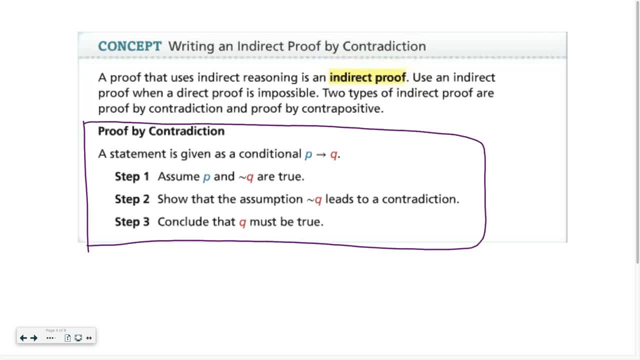 The really, really important stuff is right here. So when you write your proofs, I do ask that you actually write out step one, Like the words Write- Literally write Step one And then fill in whatever information you have. I will ask you to write step two and I will ask you to write step three. 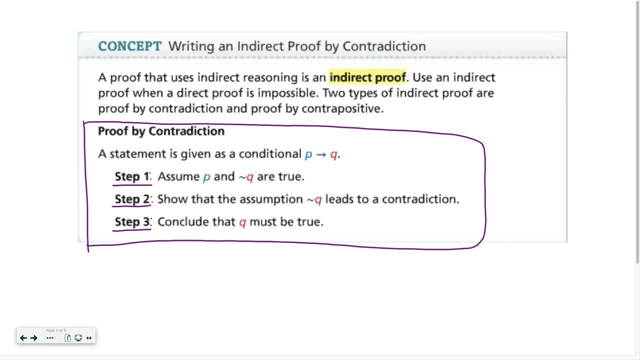 Okay, So proof by contradiction: Suppose we have a conditional: If P, then Q, Our first step in writing this proof Is to: Is that we assume that the original statement P is true And we assume that the negation of Q is true. 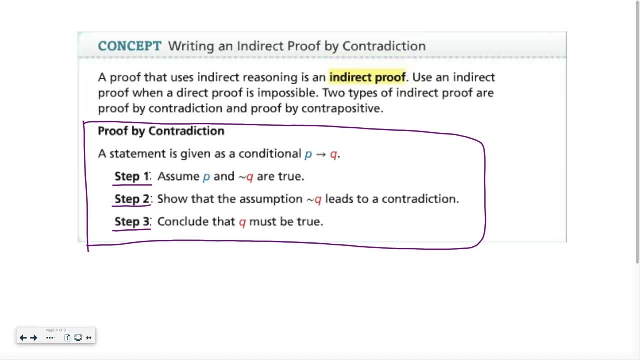 Okay, So I'll show you exactly what that looks like with an example in just a minute. Step two is that you show that if you assume that the negation of Q ends up causing a contradiction or leading to something, that isn't true, that's what goes in step two. 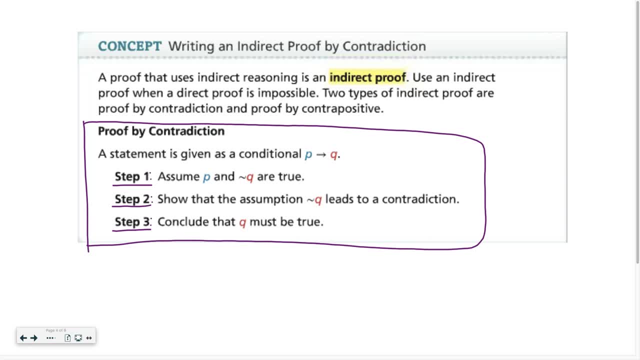 Sometimes. Sometimes it's calculations, Sometimes it's definitions, So it's just words. It depends on the situation. Step three: You conclude that statement Q must be true. Okay, So let's talk through what this might look like. 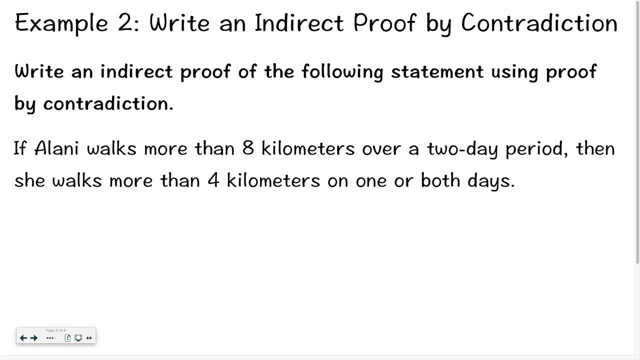 So example two: Write an indirect proof by contradiction. So we want to write an indirect proof of the following statement using a proof by contradiction And our Um Conditional- Sorry, I forgot the word- Our conditional- is If Alani walks more than eight kilometers over a two-day period. 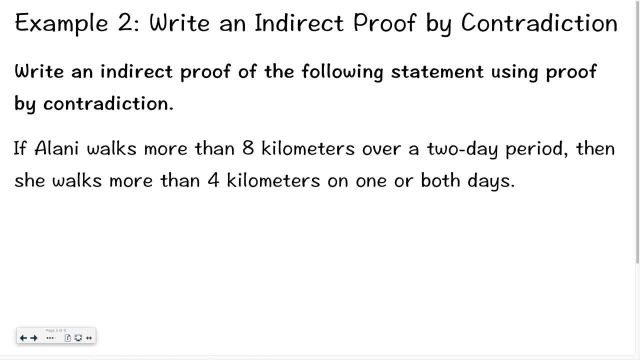 then she walks more than four kilometers on one or both days. So our step one, Write out step one And remember. this is where you assume that if P, then not Q, is true. Okay, So I'm going to say assume, 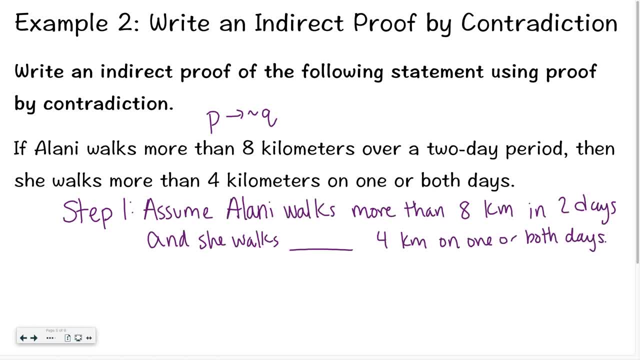 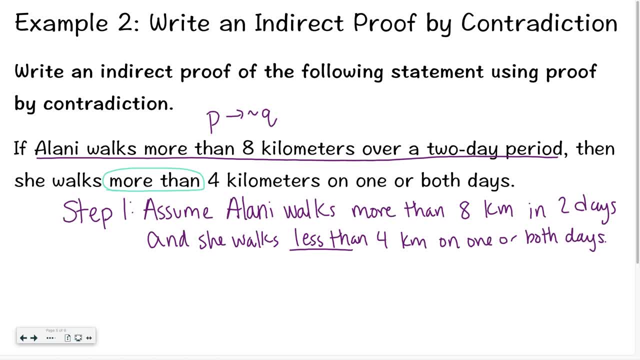 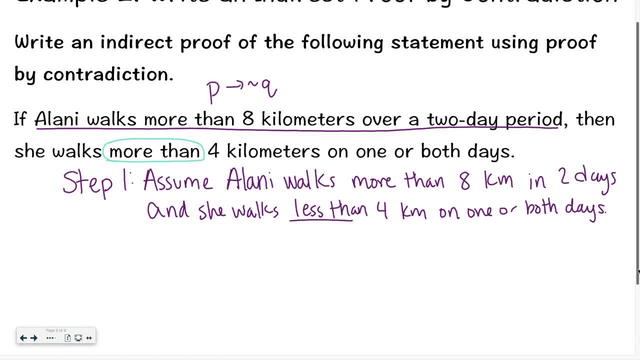 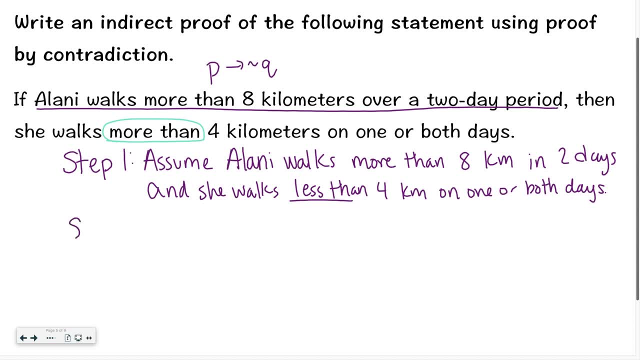 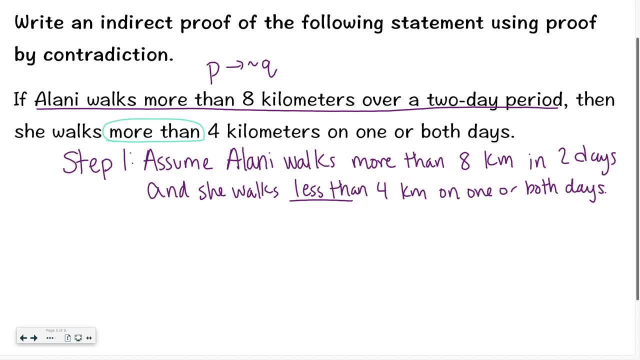 Actually I'll do step two in another color. So step two, All right. So let's look at the Q statement. She walks less than four kilometers on one or both days. So less than four Means that four is not included. 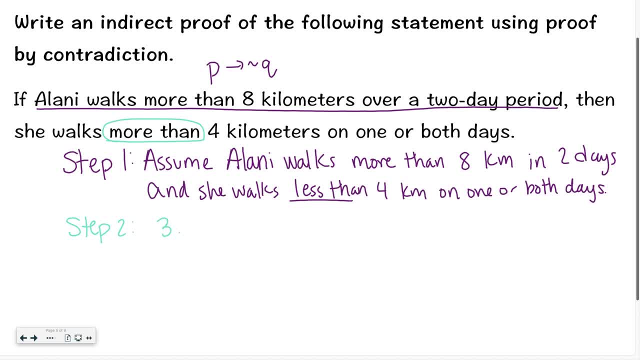 So I could say like 3.9 and I could say 3.5.. Those would both be less than eight kilometers um for the two days And if I did that I would end up with 7.4.. Even if I did 3.9 plus 3.9, I ended up at 7.8.. 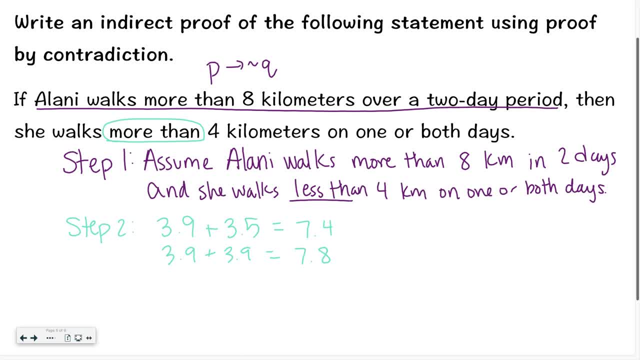 Okay, Okay, Okay, Okay, Okay. And both of those numbers. it doesn't matter what two numbers you plug in, you're never going to get to more than eight kilometers. So you can see that these two items are both less than eight. 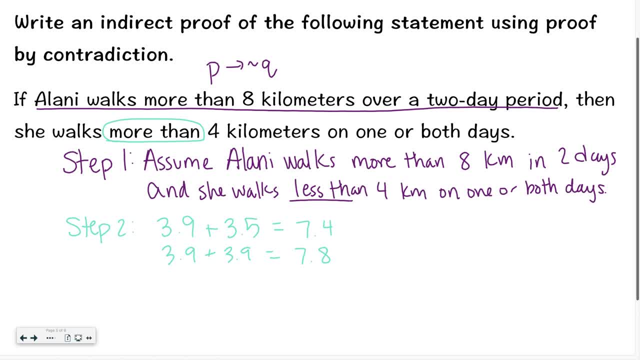 And I can actually write that a little nicer for you guys. I can say 7.4 less than eight, 7.8 less than eight. All of those numbers are going to be less than eight. You can write this out with variables to be a little more specific. 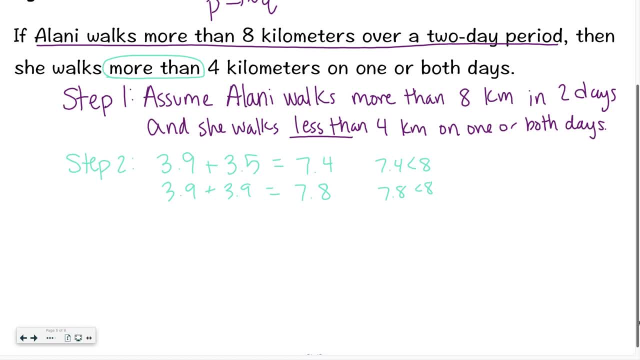 I'm more focused on you guys learning how to do the different steps than getting super complicated in those calculations. Okay, So then step three. I've done some calculations to prove in step two. So step three: this is where I kind of write a couple of sentences to show that the assumption 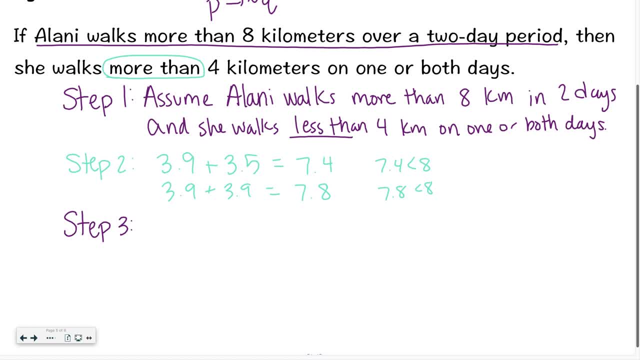 the proof by contradiction led to a contradiction, hence contradiction: proof by contradiction. So our original statement must be true. So in step three, I wrote: since our assumption in step one led to a contradiction of the hypothesis, the original statement must be true. 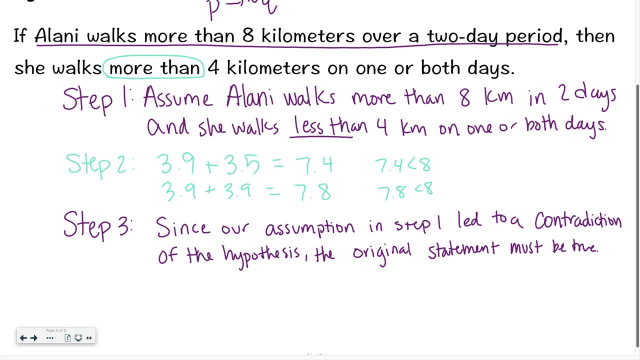 All of your proof by contradictions, I'm okay with them ending with some sort of form of that. If you want to be a little more specific and include details from the specific problem, that's fine. But I'm okay with this just being kind of an introductory proof by contradiction, indirect proof, okay. 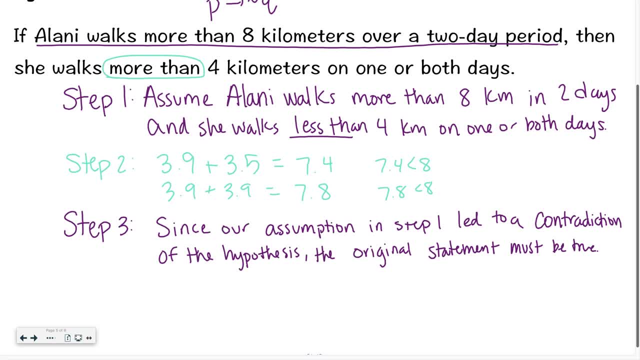 You can do a generic step three, Since our assumption in step one led to a contradiction of the hypothesis. the original statement must be true And that contradiction of the hypothesis. you might be a little confused by what that means, but that's what we did in step two. 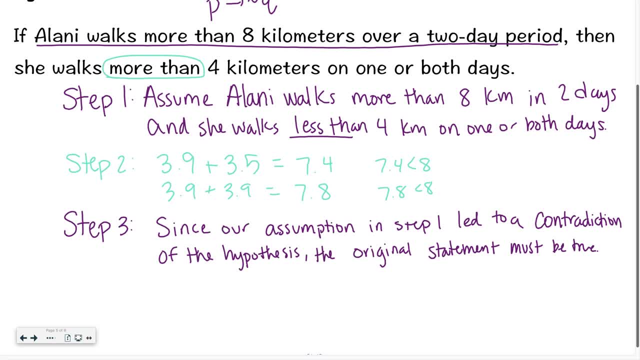 We showed that the step two, those calculations, that's what we did in step two. We showed that the step two, those calculations, that's what we did in step two. We showed that the step two, those calculations, they didn't hold the hypothesis true. 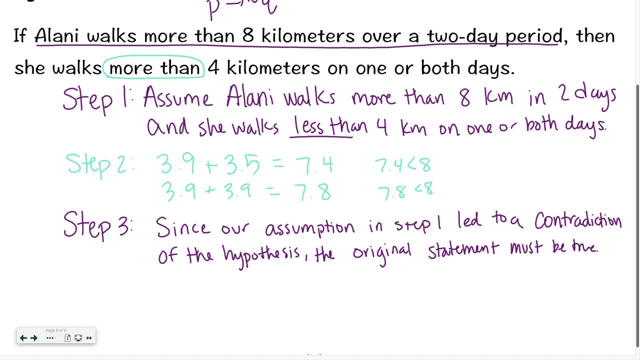 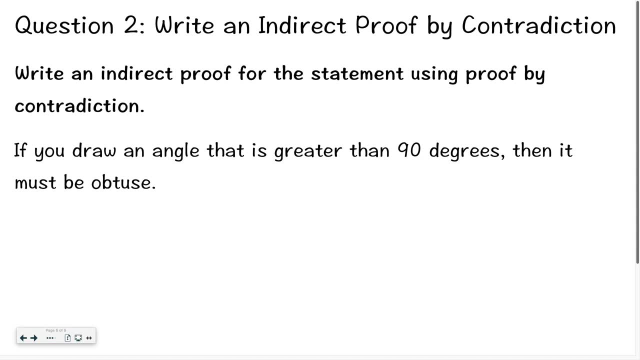 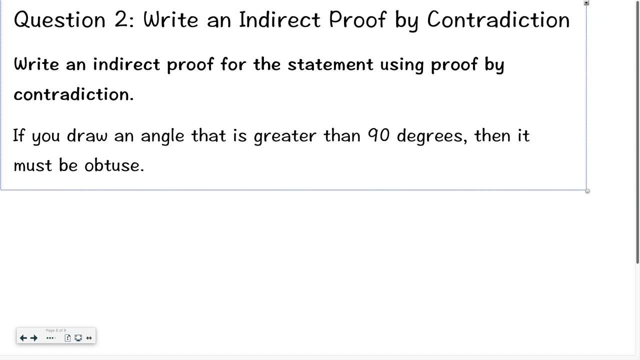 They weren't more than eight kilometers. okay, I want you to try to write an indirect proof by contradiction. Remember your step one, two and three And try to write it down on your paper and then pause your video. And try to write it down on your paper and then pause your video. 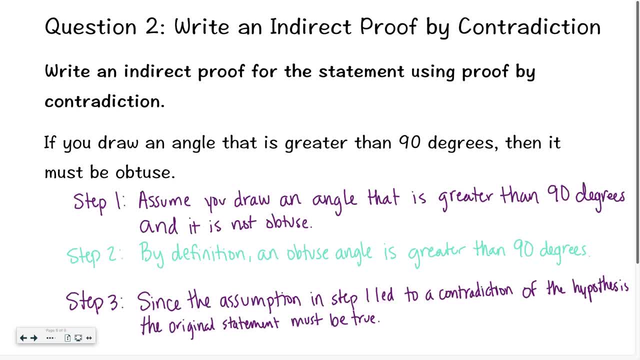 And, once you've written it down, check your answer. okay, Hopefully you ended up with something that looks like this. Hopefully you ended up with something that looks like this. Step one: you made an assumption that you draw an angle that's greater than 90 degrees, and it is not obtuse. 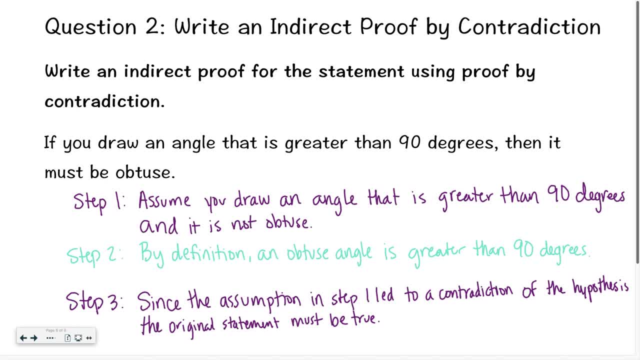 Step two, you can say: well, by definition, an obtuse angle is greater than 90 degrees. okay, So that means in step three, you can just say: since our assumption in step one led to a contradiction, Meaning it contradicted the very definition of obtuse, 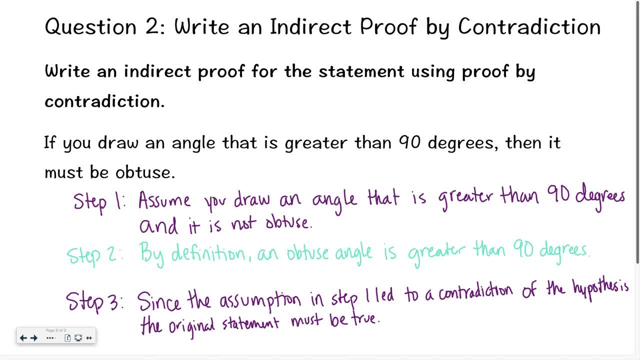 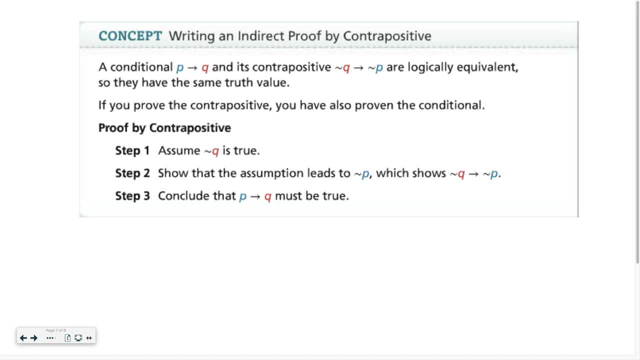 So since it led to 90 degrees and it is not obtuse- led to a contradiction of a hypothesis, the original statement must be true. All right. indirect proof by contrapositive: same idea but just slightly different. So we talked about contrapositives back in. I believe it was 1.5.. 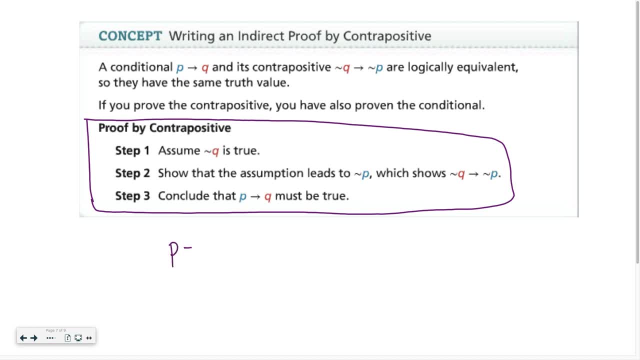 So remember we talked about all of those different. if P, then Q was our conditional. if Q, then P was our converse. if not P, then not Q was our inverse and our contrapositive was: if not Q, then not P. 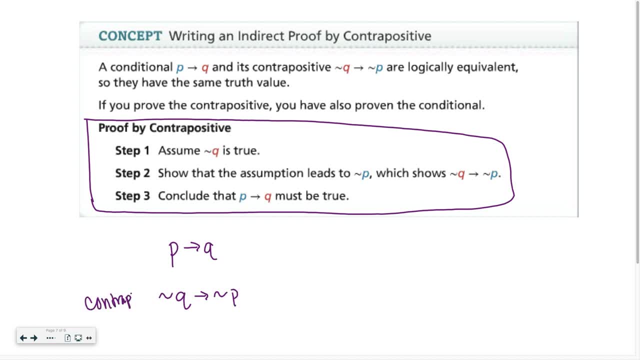 Okay, remember, that's our contrapositive. All right, so just a little background there. So step one: assume that not Q is true. Step two: show that the assumption leads to not P, which shows that if not Q, then not P. 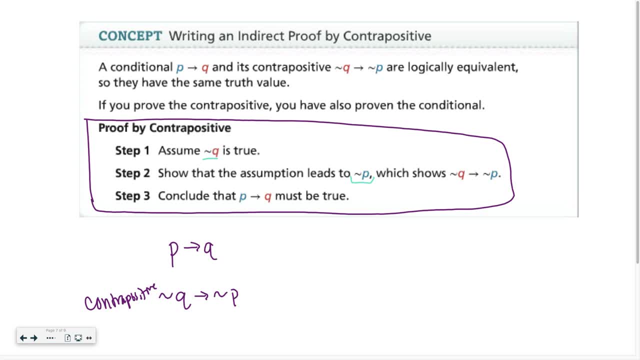 So then you're able to conclude that if P, then Q must be true. Now, if you remember going back to the conditionals and the contrapositives, those two things always had the same truth value. So that's why. that is why, if you're able to prove, if not Q, then not P. 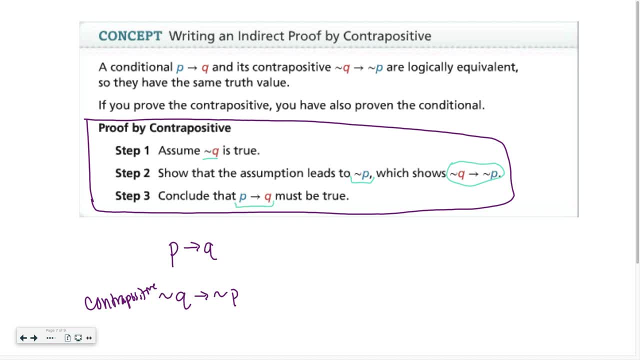 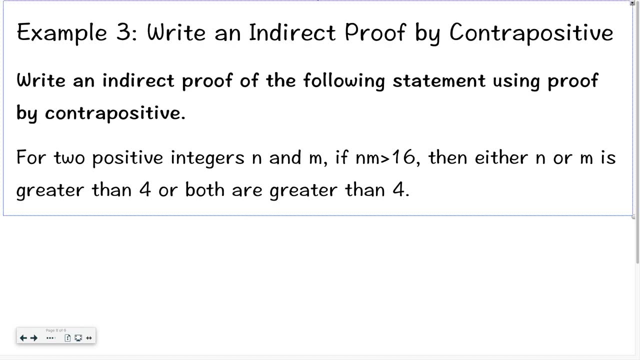 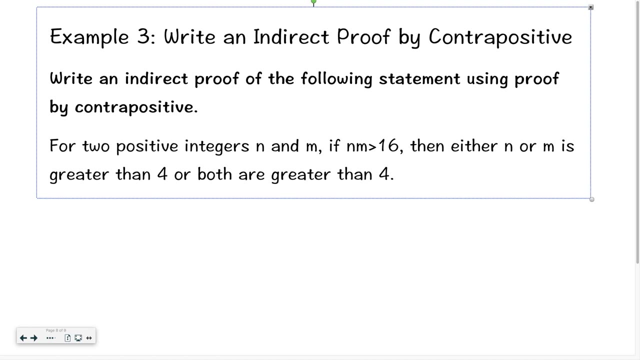 that proves, if Q, Because they have the same exact truth value. All right, so now let's talk through the indirect proof by contrapositive. So our indirect proof by contrapositive. remember, we're still going to do those three different steps. 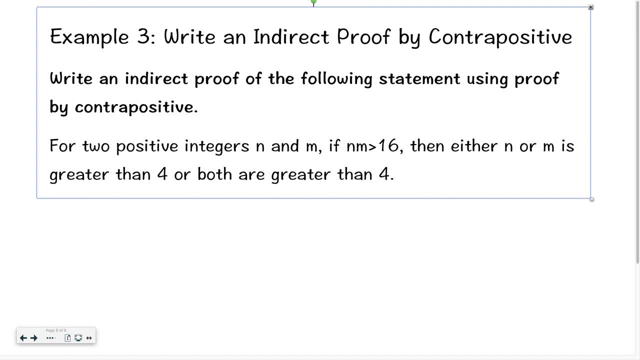 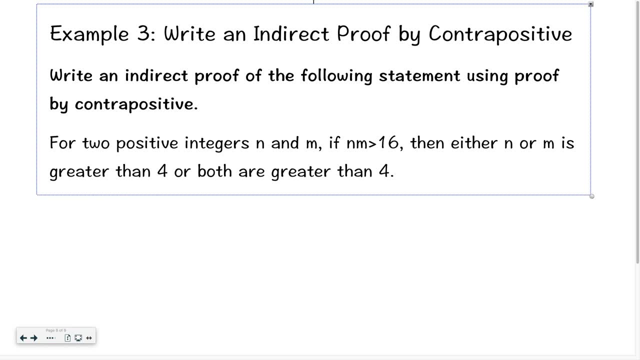 And our first step, remember, is to show if not Q, or assume not Q. So let's start. So let's start by just identifying the P statement and the Q statement. So P for two positive integers, N and M. 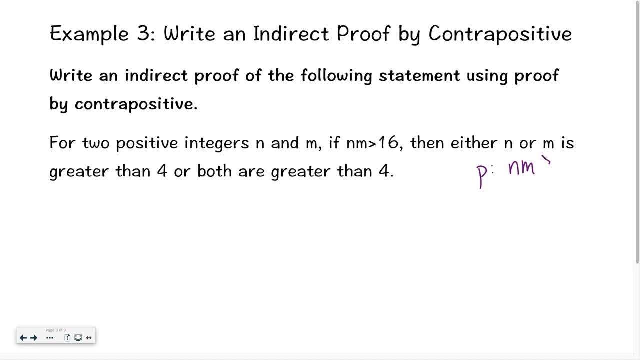 if NM is greater than 16, so that's going to be my P statement. So my not P statement would be: NM is instead of greater than, I'm going to say less than 16. But I'm also going to include that or equal to. 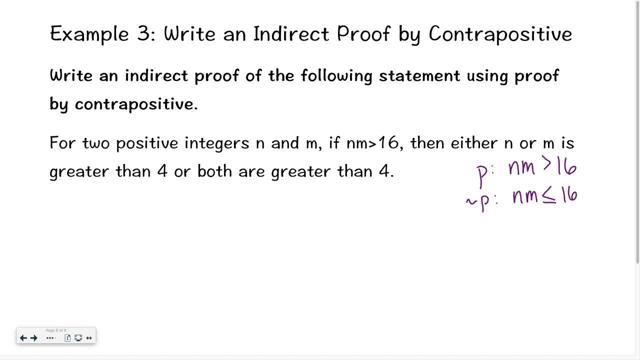 So that way the number 16 is included somewhere For my Q statement. then either N or M is greater than 4, or both are greater than 4.. So Q would be: N is greater than 4, or M is greater than 4,. 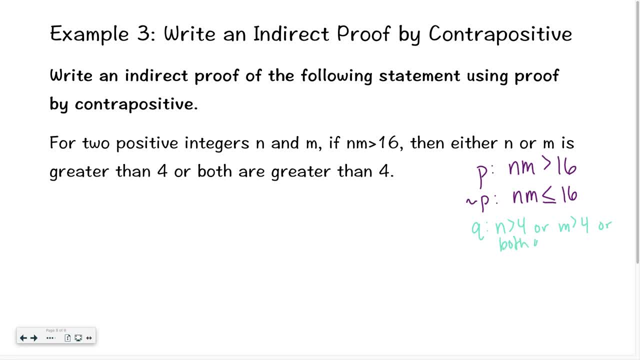 or both are greater than 4.. So my not Q would be: N is less than or equal to 4.. And so, instead of using the word or, I'm going to use and and M- sorry- is less than or equal to 4, okay, meaning they both have to be less than 4.. 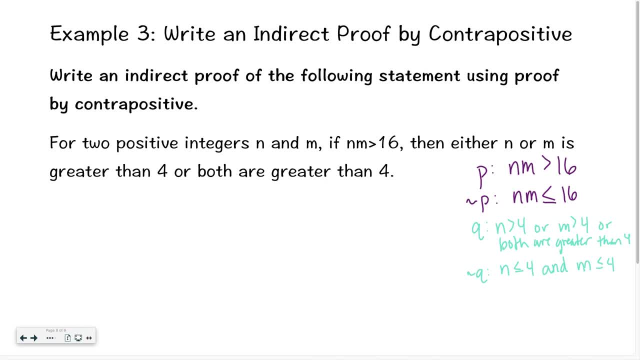 So that is the opposite of 4.. That's the opposite of what was stated previously. So step one, assume not Q is true. So we are assuming that N is less than or equal to 4, and M is less than or equal to 4.. 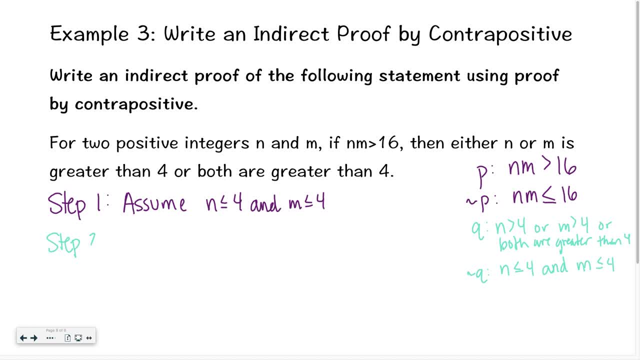 Step two: okay, so if I know that I have N is less than or equal and I am, M is less than or equal to 4.. Now, remember, I'm trying to show that step two gets me. I can somehow manipulate this step and get to my not P. 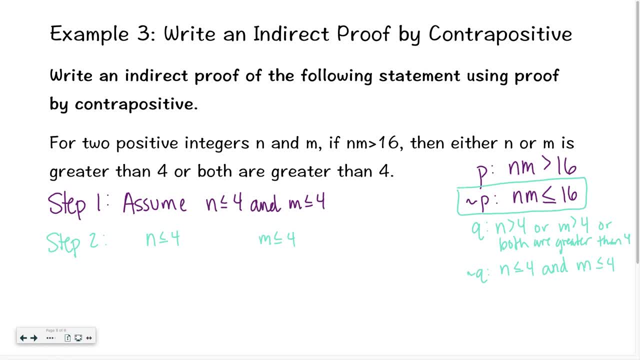 So I want somehow to get it to look just like that. Okay, so if I am trying to get these two inequalities to look like that not P statement, if I look the left side of the not P inequality is NM. So how can I change this first inequality here to have an NM on the? 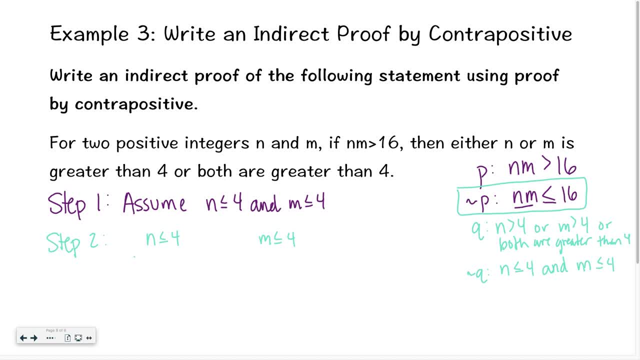 left-hand side, I'm going to multiply by an M, So I'm going to multiply by M on the left side. That means I also have to multiply by M on the right side, Because as long as you multiply by the same amount on each side, you're okay. Now, if I look at this right-hand inequality- and I want that to- 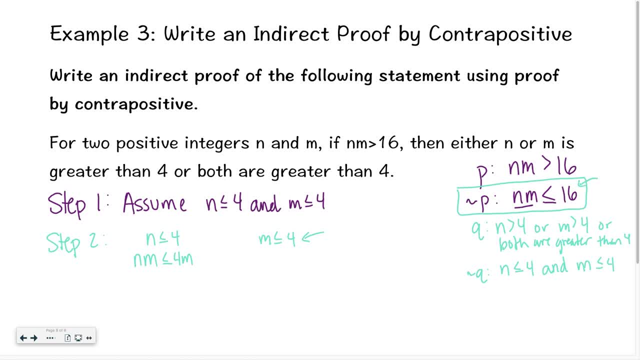 look like the right-hand side of my- not P- inequality: I have to get a 16.. So what do I have to multiply both sides by in order to get a 16? in one of those places, I have to multiply by a 4.. So if 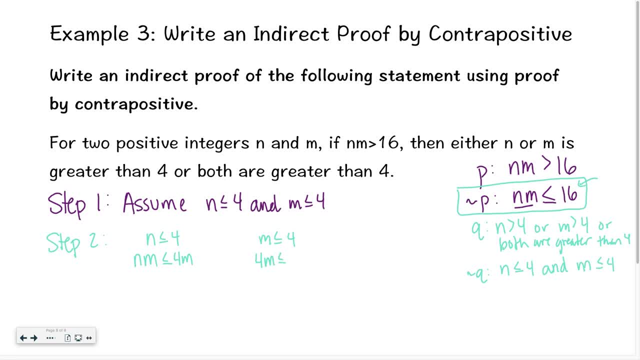 I say 4 times M is less than 4 times 4, which is NM, which gives me 16 on that right-hand side. So now if I look at these I could say NM is less than or equal to 4M. And then look, 4M repeats. So I can just say 4M is less than or equal to 16.. But the 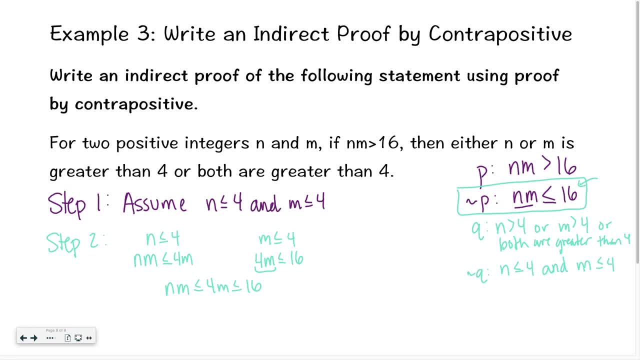 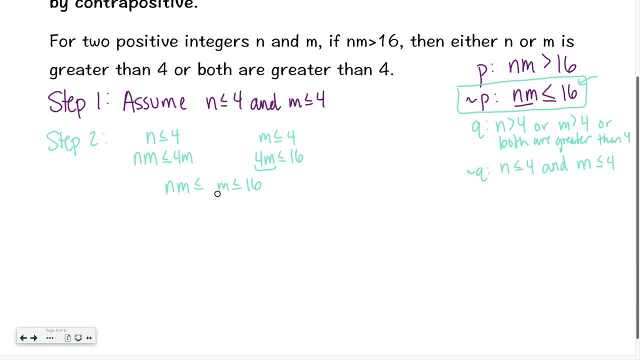 not P statement doesn't have that 4M anywhere, So what I can do is get rid of it. So if I erase it, I erase that 4M. I have two inequalities now facing the same exact way, So I'm just going to. 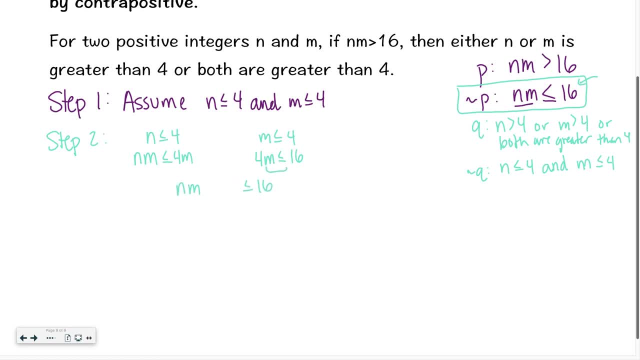 erase one of them And if I look that did not move like I thought it would, I can move that NM over. So I just used algebra to kind of manipulate those two inequalities in order to get them to match that not P statement. And since I was able to get it to match, I'm going to get it to match. 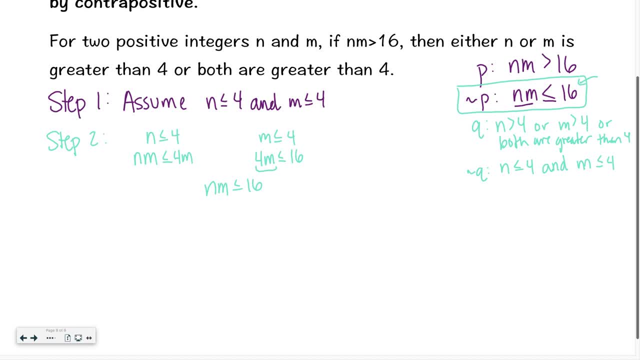 So I'm going to get it to match. And since I was able to get it to match, I'm going to get it to match the not P statement. That means I was able to get it back in the form: if not Q, then not P, And. 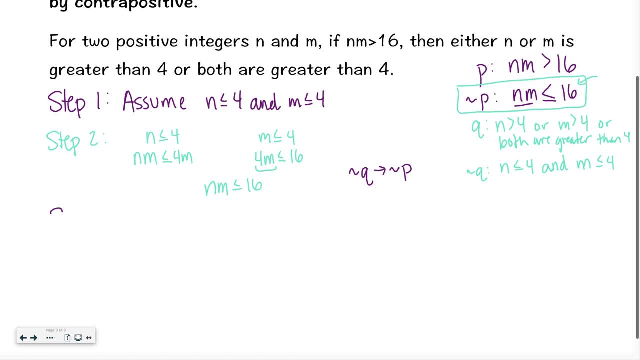 since I was able to get it back in that form, my step three. I am ready for now, So I can say step three. I can say something like: since step two gave us the contrapositive, we can conclude that the original statement less than or equal to 4M is less than or equal to 4M. And since I was able, 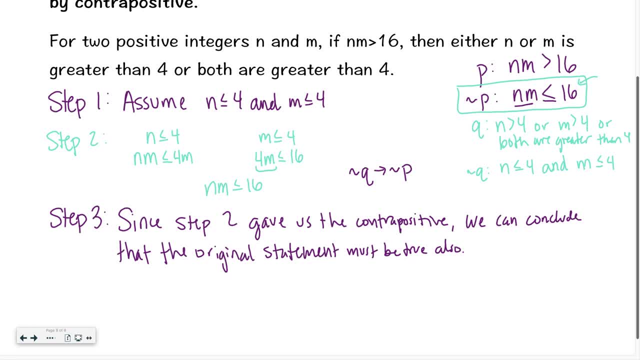 to get a single word. that must be true also. Okay, We can conclude that the original statement must be true also. Okay, We can conclude that the original statement must be true also. Alright, Now I want you guys to try, just like you did with the proof by contradiction. Try this: 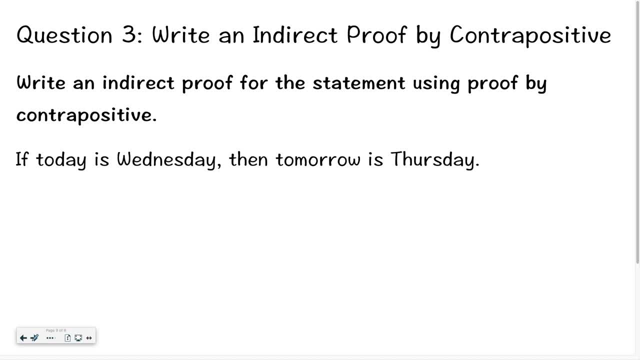 proof by contrapositive on your own And then compare your answers to mine. Good luck, Hopefully. your step 1 looked similar. you assumed tomorrow is not Thursday. Step 2, if tomorrow is. your step 1 looked similar. you assumed tomorrow is not Thursday. Step 2, if tomorrow is not. 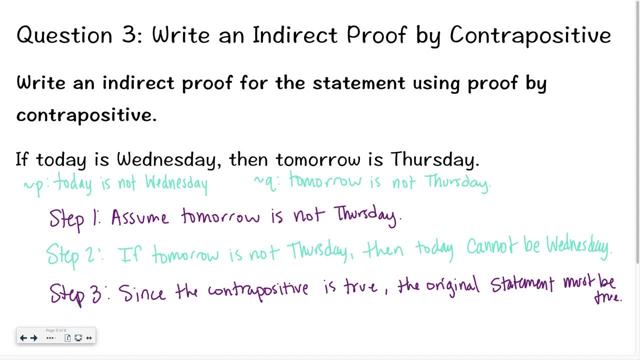 Thursday. so I started with that, not Q statement. so just thinking about that, if tomorrow is not Thursday, then today cannot be Wednesday. and that right there, just thinking about that, if tomorrow is not Thursday and I'm thinking to myself, well then today can't be Wednesday. that, right there, actually gave me the 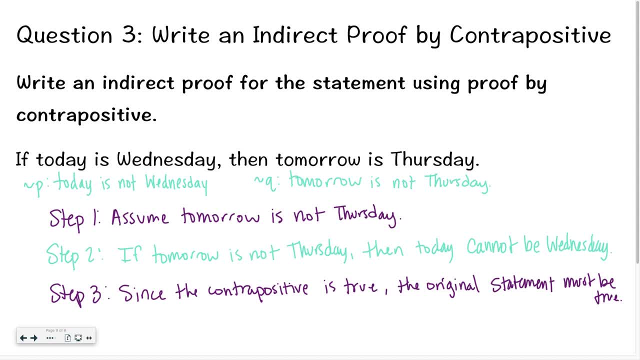 contrapositive. that is the contrapositive, which means I am ready to move on to step three. just since the contrapositive is true, the original statement must also be true. okay, I know these are gonna take some practice and maybe be a little frustrating for you guys, but remember, I'm here to help and